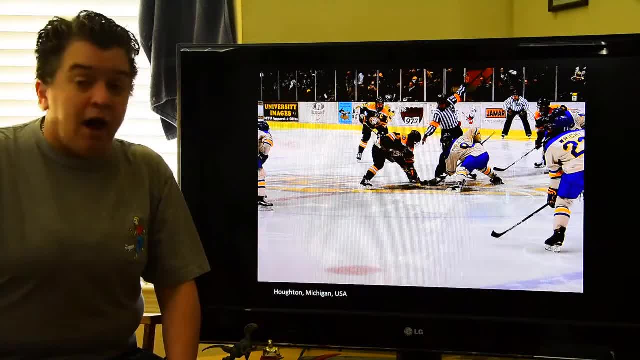 up stories I also like sports a lot I love watching a lot of sports I also like sports a lot I love watching I also like sports a lot I love watching 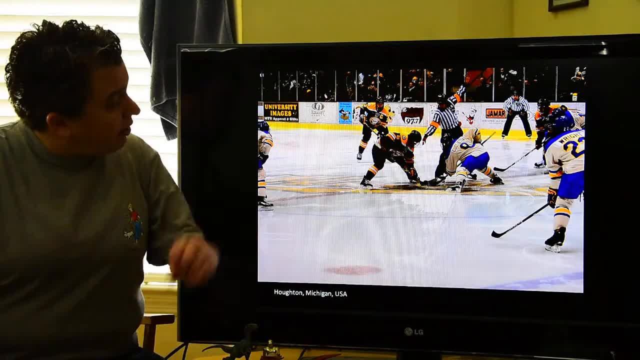 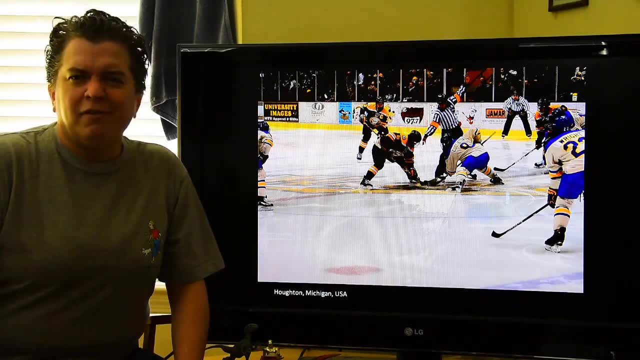 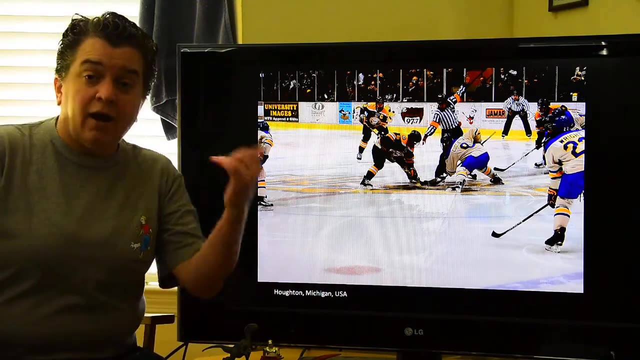 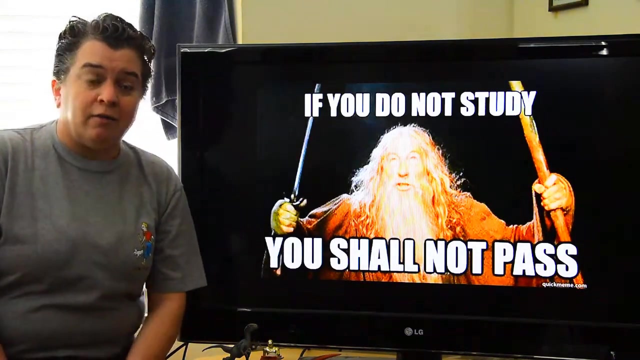 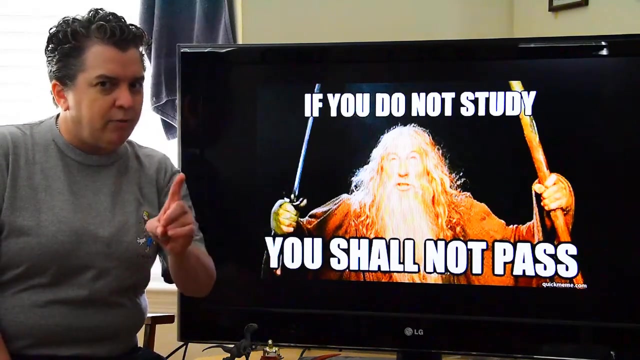 American football and hockey that's actually Michigan Tech playing hockey there and so I'm hoping there's gonna be a football season because I'm gonna be really bored if I can't like yell at the refs about plays and calls and things but anyway I like sports as well all right now what about the class well it's a science class so it is gonna be hard and so take Gandalf's advice here you know if you do not study you shall not pass but remember I am here to help you right so if you're confused about 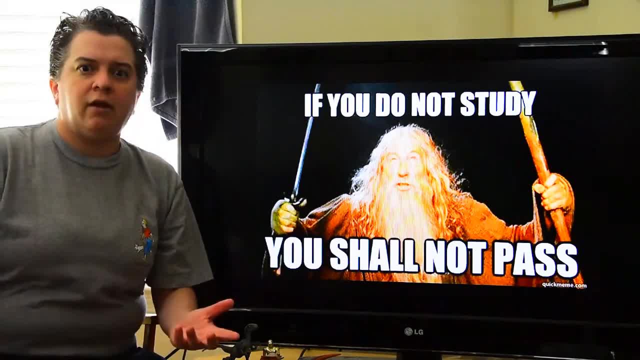 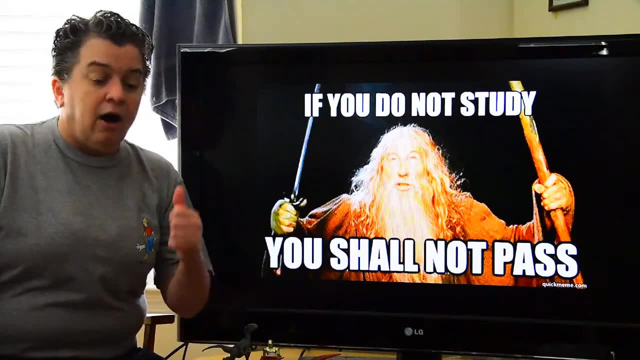 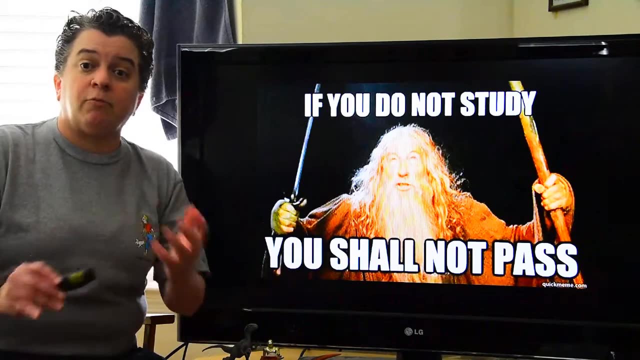 something or you don't understand one of the activities please get a hold of me and tell me that you're confused so I can help you with that on d2l I'm gonna post my my cell phone number as well as my personal email so if for some reason you can't get through to me using d2l or your Lone Star account you can always shoot me an email. 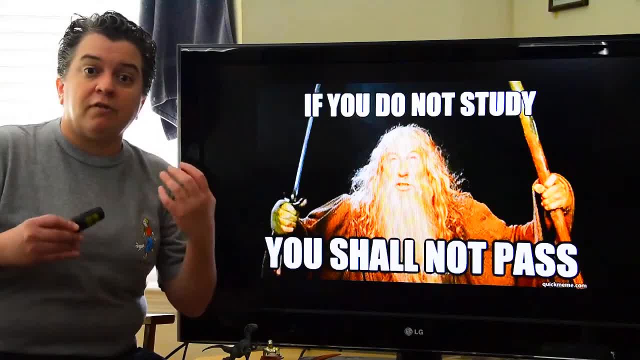 a text give me a call you can email me just let me know that you're having trouble or are confused because my job is to try to help you understand the 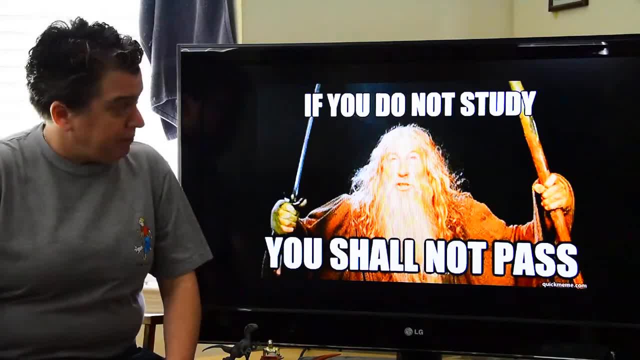 material so don't hesitate to contact me so let's talk a little bit about what 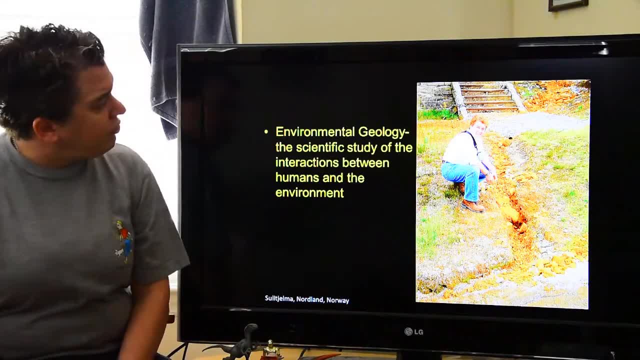 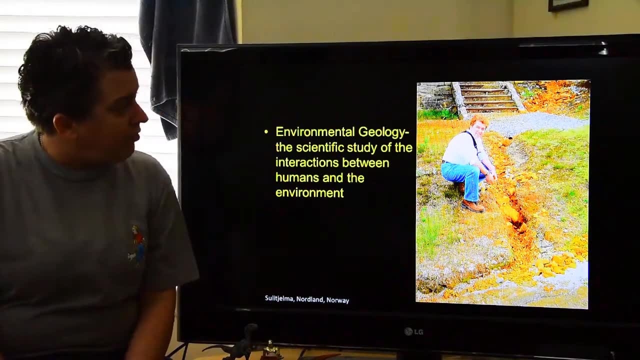 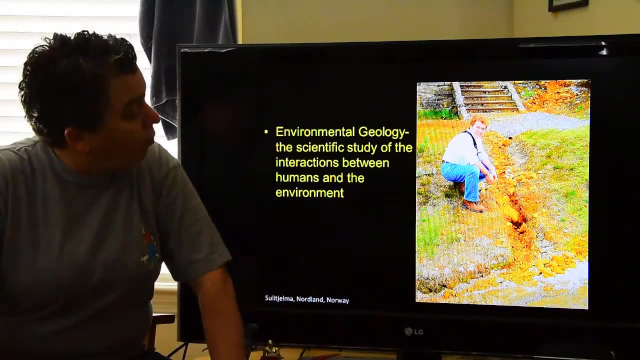 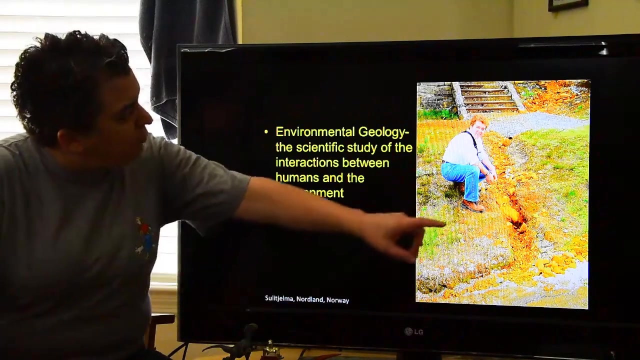 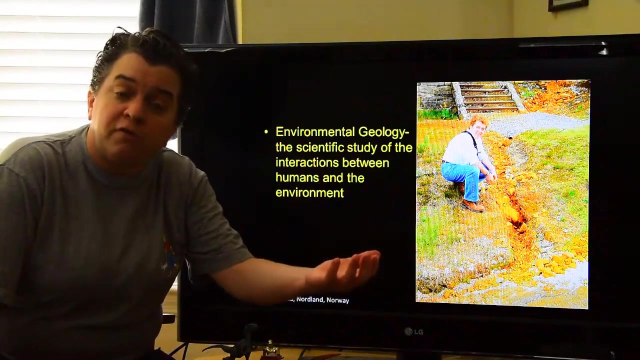 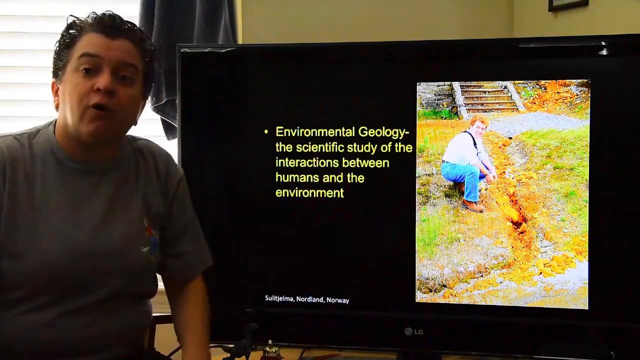 we're gonna spend the rest of the semester studying environmental geology this is the scientific study of the interactions between humans and the environment that's actually what I'm looking at right here in this illustration this is the scientific study of the interactions between humans and the environment that's actually what I'm looking at right here in this illustration this is a an old mining area in northern Norway and we're taking a look at how the minerals that were exposed there when they degrade when they decay basically because of being exposed to the atmosphere and water they turn into an acid and that's what we're seeing in this weird colored rock right there so 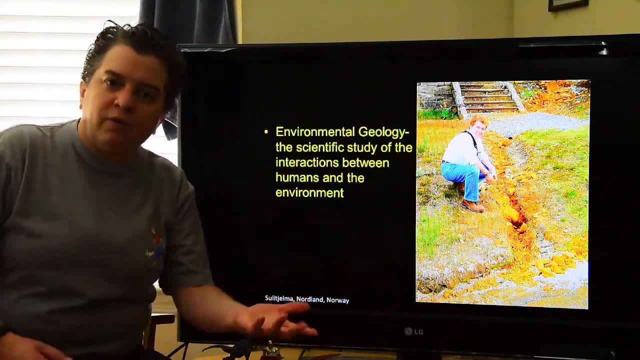 I'm taking a look at how humans have interacted with the environment there you 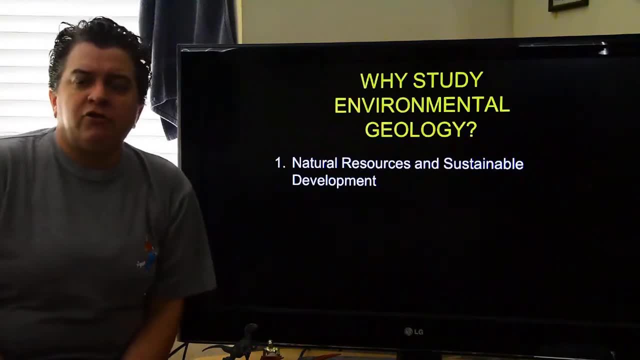 know why would you study environmental geology I'm hoping that a few of you sitting out there are saying I'm studying this because I want to be a 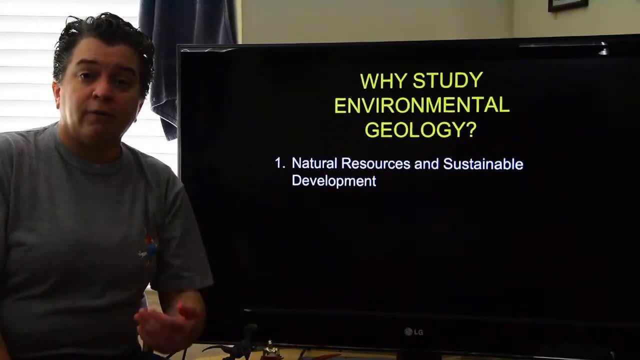 geologist and that would be fantastic it's a great career but you might also just be sitting there saying well I need a science credit and I didn't want to 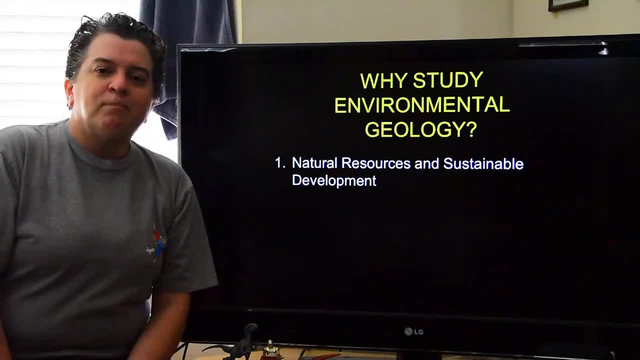 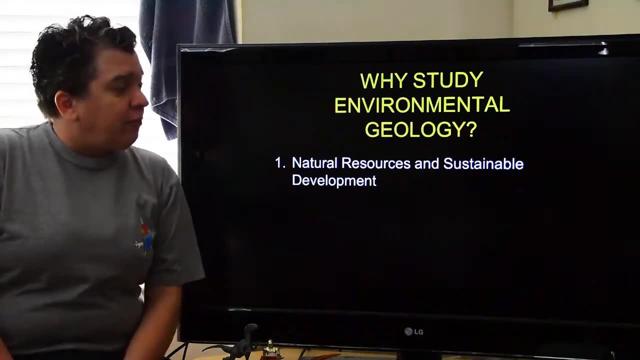 take physics then that's okay too but there are some real reasons to study environmental geology and one of those is natural 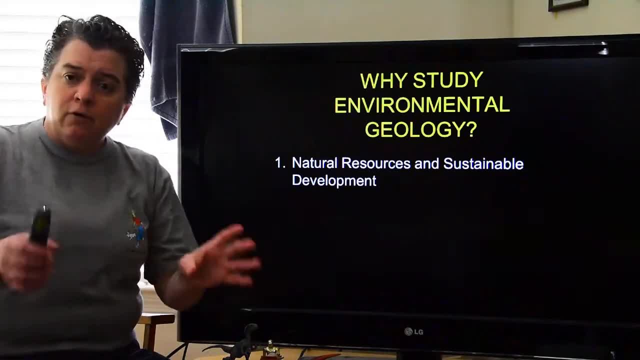 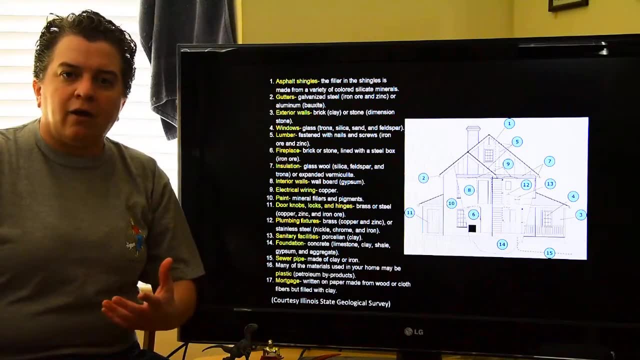 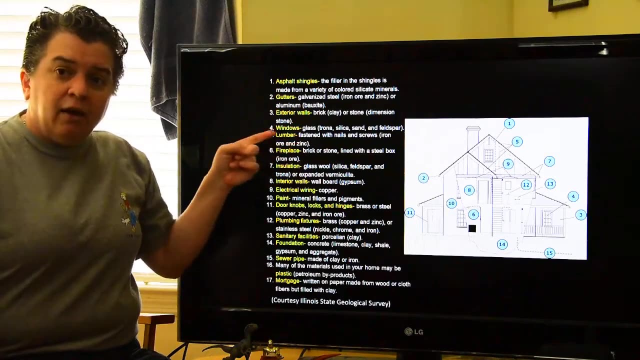 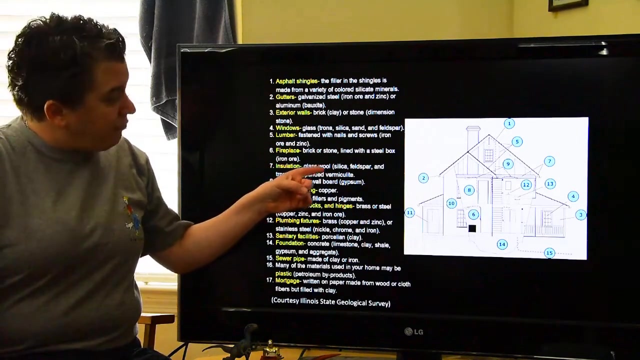 resources and sustainable development if you look around you're gonna see that much of your house is made out of things we get out of the earth and in fact this is kind of a typical house the parts that go into it and it's explaining where we get this stuff from for instance you know you have the the insulation is something called glass wool that's made from silica basically quartz and feldspar you have the electricity and you have the energy from a carbon fiber system that's made from silicon basically quartz and feldspar you have the electrical energy from the energy from the PVC. 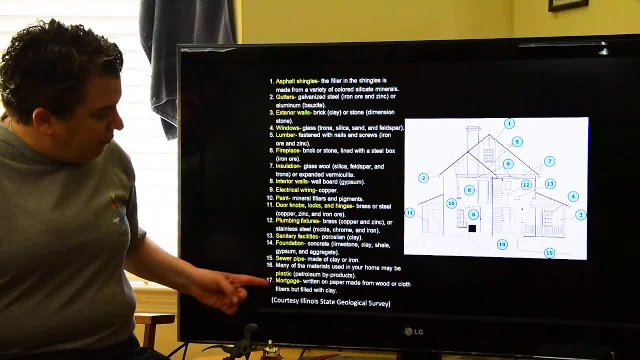 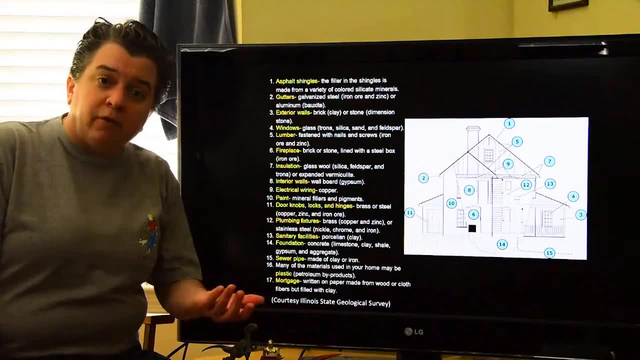 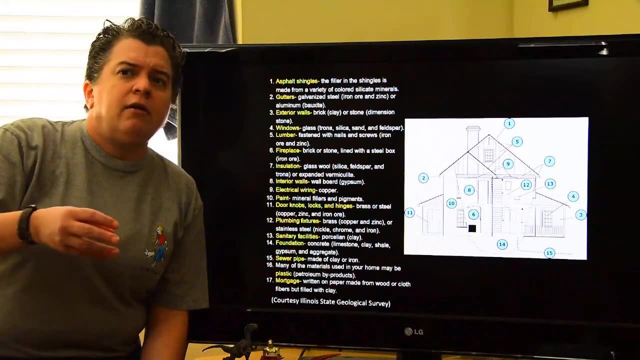 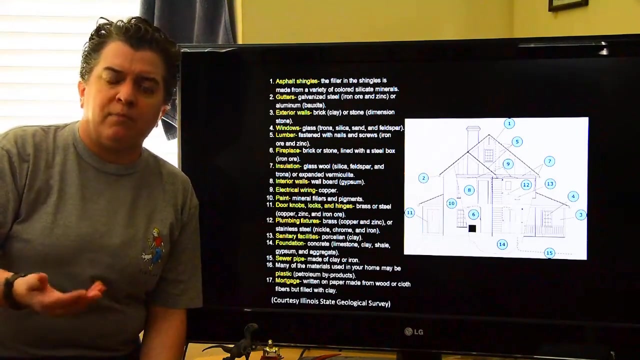 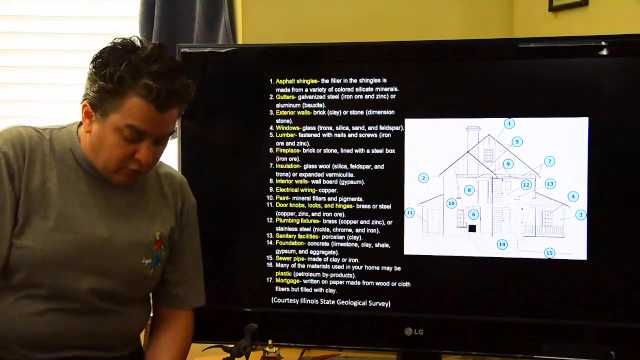 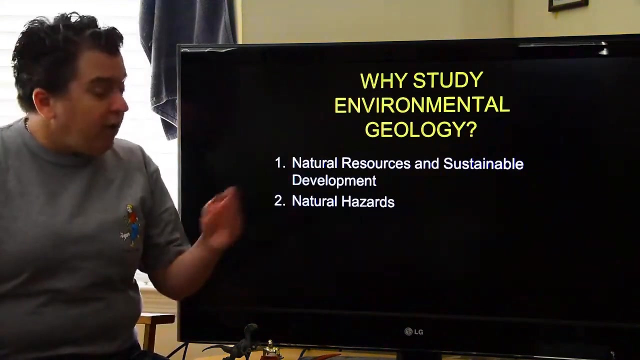 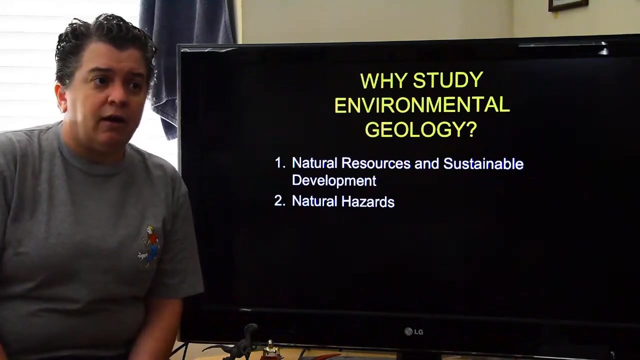 wiring, made from copper, even paper. The binders that hold the wood pulp together are different kinds of clay minerals. And so we use minerals every day for all kinds of things and we need to make sure that we use them wisely. That's the whole concept of sustainable development. Extracting these things out of the ground with the minimal amount of impact to the environment, and later on in the semester we're going to learn more about that in detail. We also study this because of natural hazards. We have all kinds of natural hazards that affect us, hurricanes and floods and wildfires and earthquakes and volcanic eruptions and all kinds of things like that. 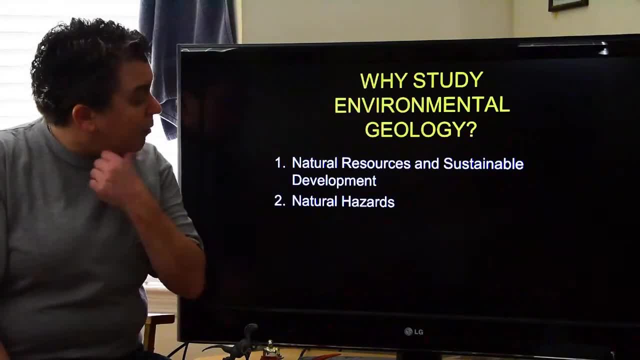 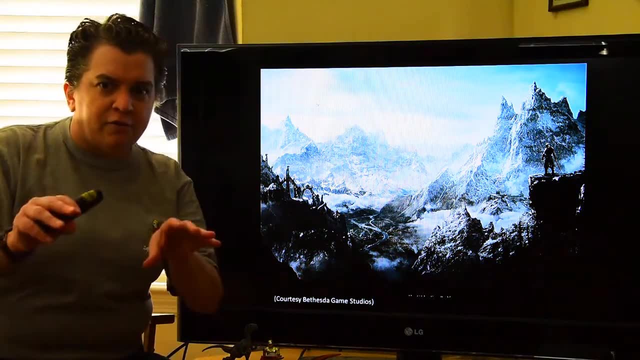 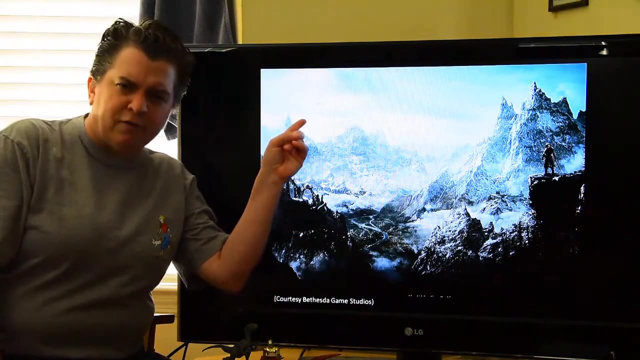 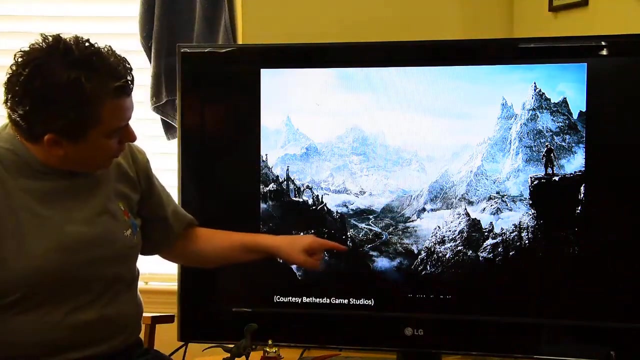 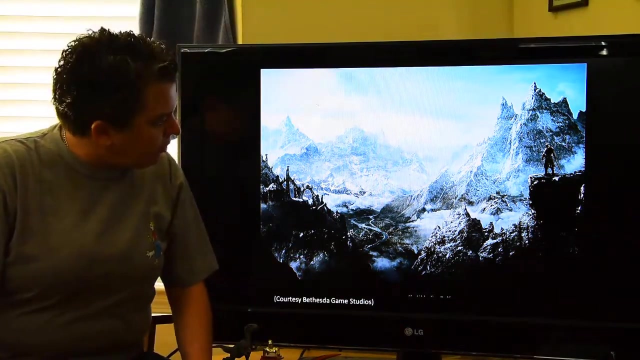 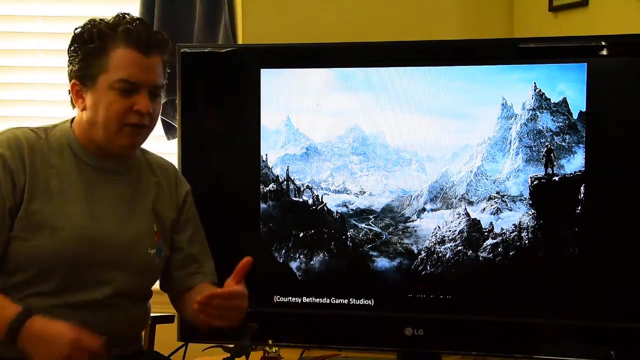 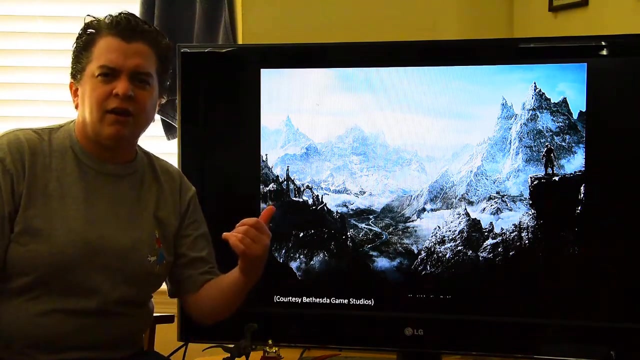 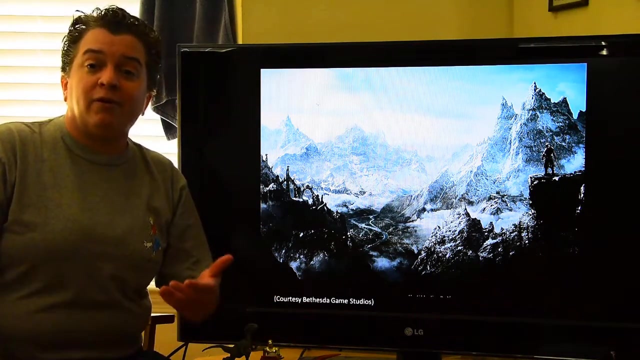 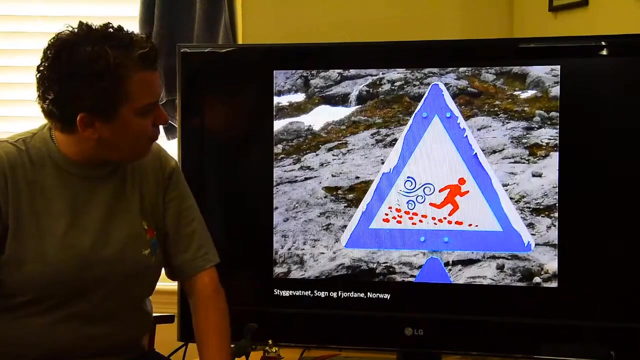 So in any case we're going to learn about natural hazards. And I gotta tell you a funny story about natural hazards and the way geologists look at the environment. If any of you guys play video games out there you might recognize this. This is not a real place. Real places do not have dragons flying around. This is Skyrim and I was playing this once and I was standing pretty much where this dude's standing here. I was looking down into this valley. There's this nice little river there in this little town called Riverwood. And when I was first playing the game I looked down at that town sitting right on the edge of this river and I was like man that's a terrible place to build a town when in springtime when the snow melts it's gonna flood. And my husband was like why do you care? The dragon's gonna eat them. But anyway geologists look at the landscape and we don't just see pretty places we also see some of the hazards of these places. And hopefully at the end of the semester you guys will be able to do that as well. So I hope you guys enjoyed this video and I'll see you guys in the next one. 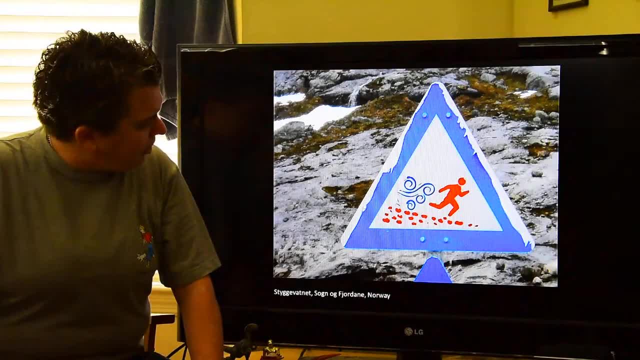 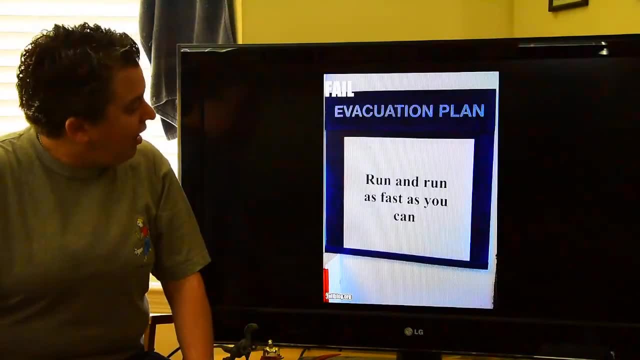 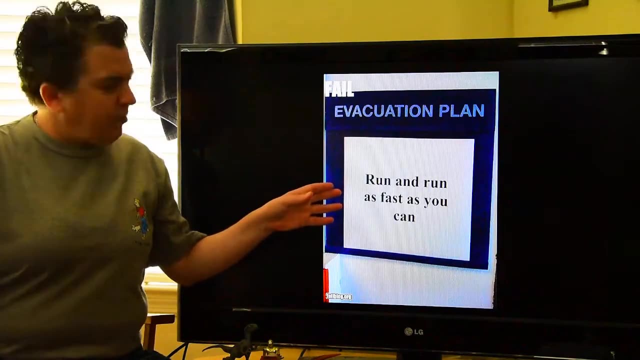 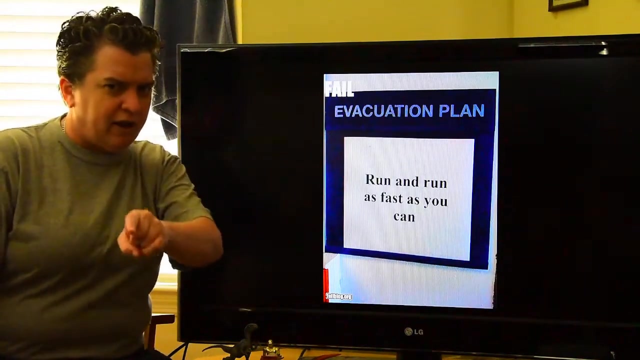 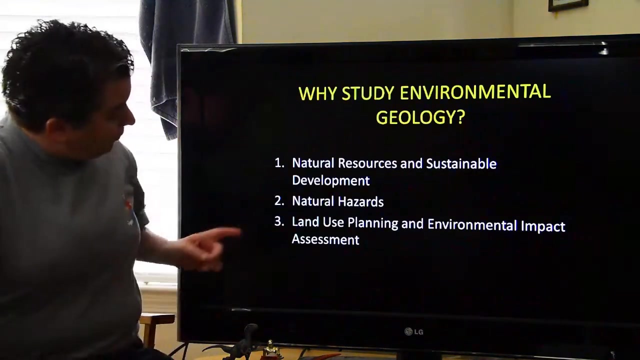 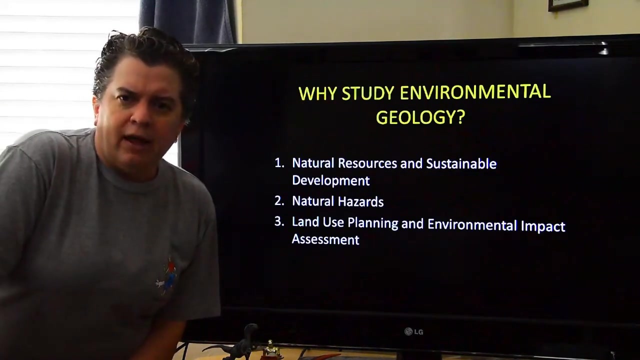 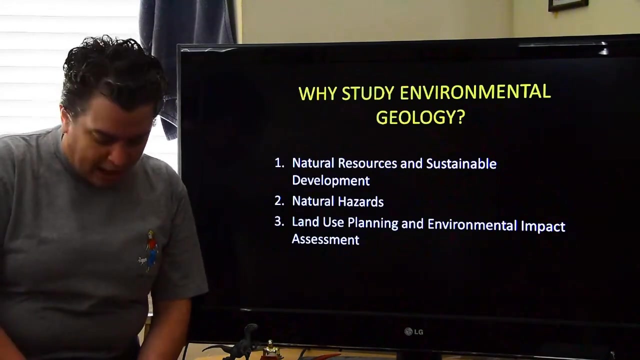 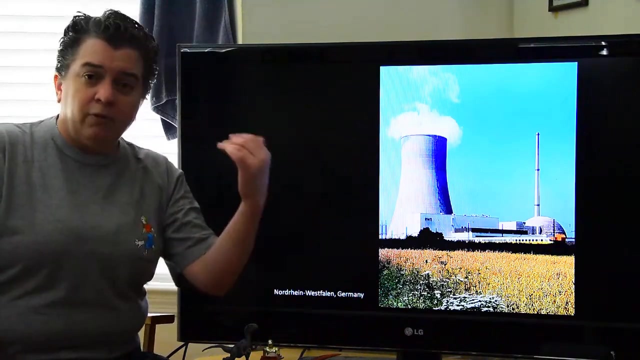 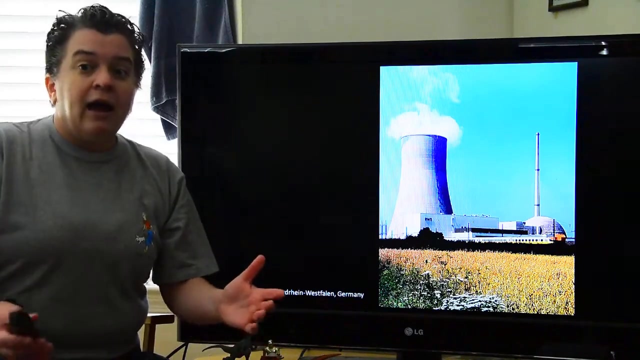 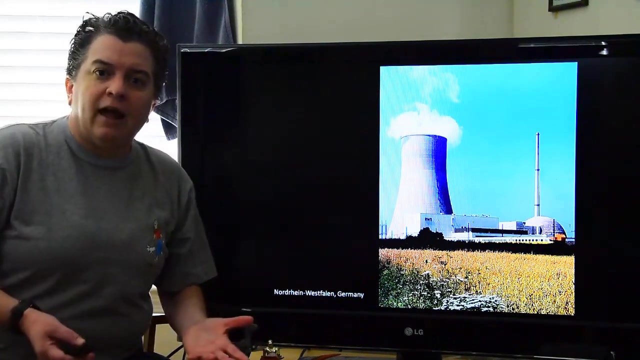 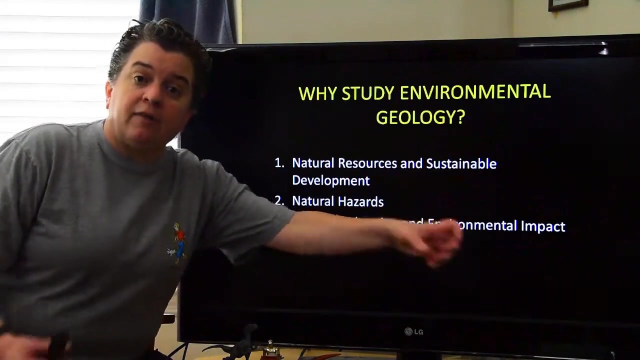 I also collect weird signs. This is a I think flash flood sign. It's little red dude running from something. And you know when it comes to natural hazards it is always good to have a plan like this. I mean it might be 12% of a plan but at least it's some percentage of the plan right. So just remember natural hazards always have a plan for them. Alright let's talk about other things we need to study this semester. Land use planning and environmental impact assessment. You know not every place on earth is a good place to build your house or a nuclear power plant or something like that. We might have something like this nuclear power plant. This is in Germany. It's in a relatively safe place but you wouldn't want to build something like that say I don't know in California on the San Andreas Fault. That might be a bad idea. And so what we're gonna learn about is how different places, and different parcels of land are useful for different things. Because you know either the impact that we would have on the environment or the impact that the environment would have 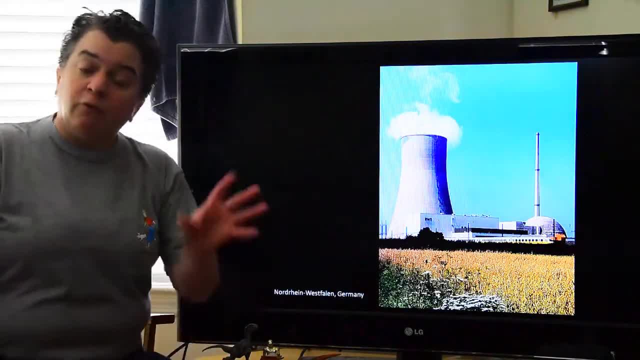 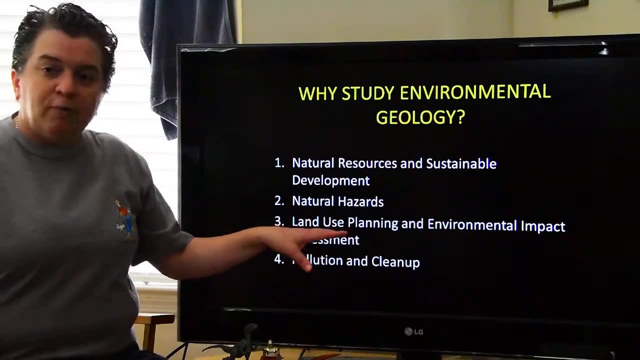 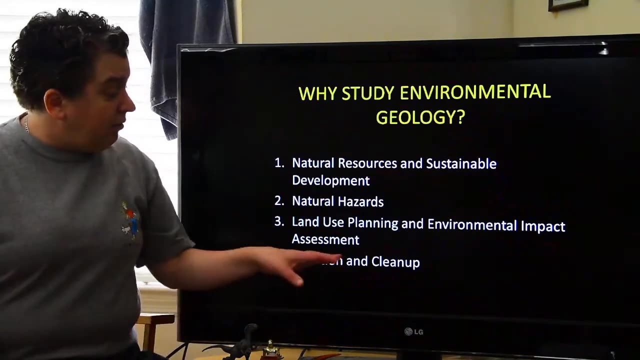 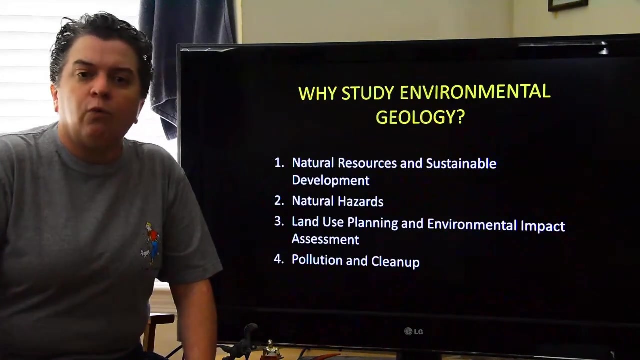 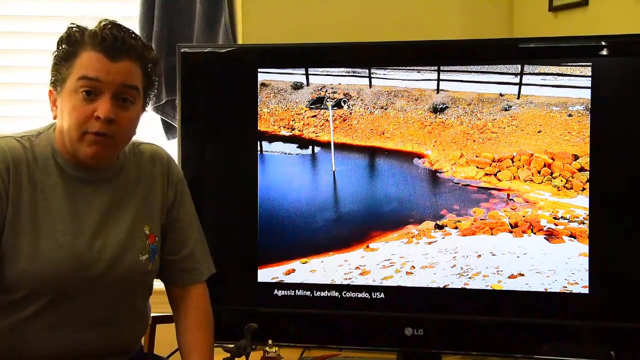 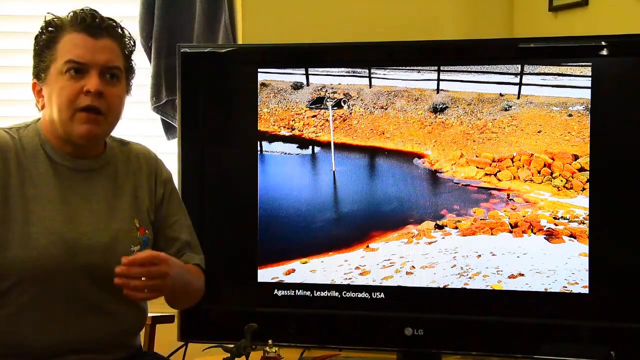 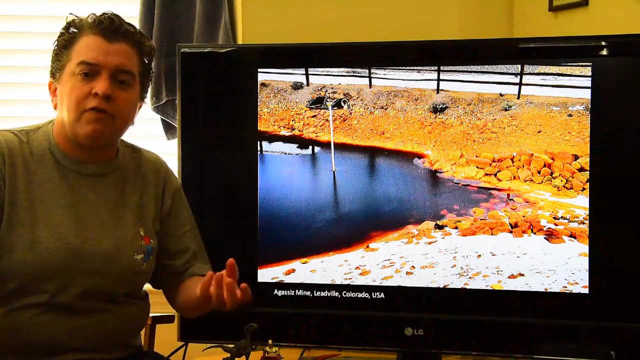 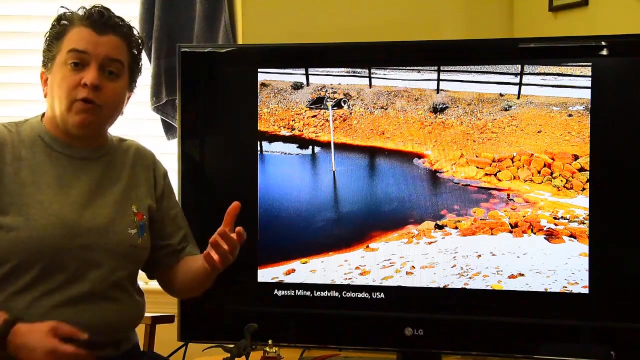 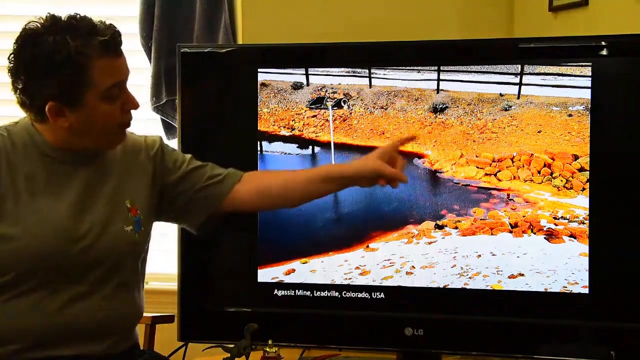 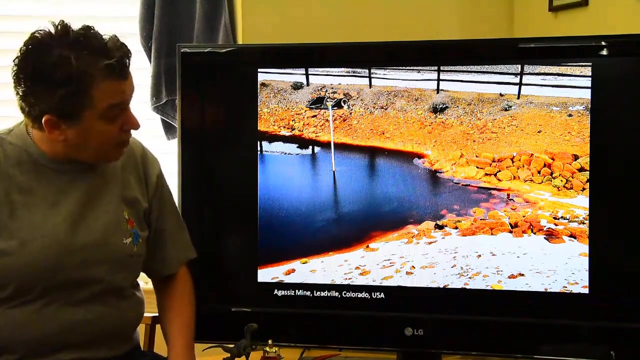 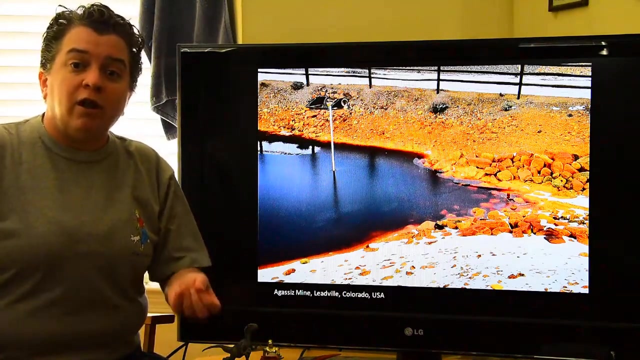 on us when we build in that location. And we'll look at that later on in the semester as well. Now of course we're not perfect. We might try to be careful about our land use planning we might try to do sustainable development but accidents do happen and we're going to have to clean those up and so we will also talk later in the semester about different types of pollution and what we can do to end that and clean it up this is an example of a type of water pollution this is in Leadville Colorado now Leadville they extracted minerals in the late 1800s and early 1900s and there weren't nearly the kinds of regulations that there are today so one of the problems then is they got a lot of acid mine drainage where the minerals the specific type of mineral they were extracting reacts with water and turns to acid and that's why we have this very strange colored water there you would not want to use acid water if you don't want to use acid water if you don't want to drink that you wouldn't even want to stick your fingers in that because it is very acidic and so now today over a hundred years after they were mining in that area some geologists are left with figuring out how to clean 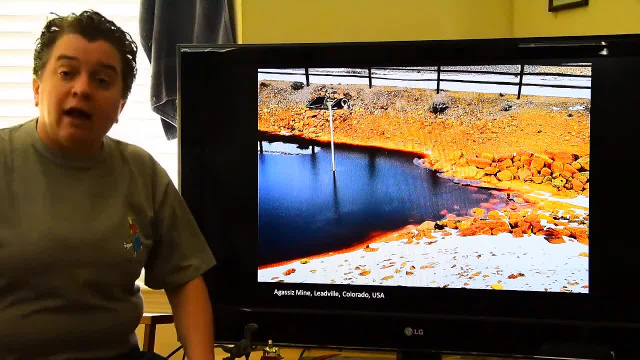 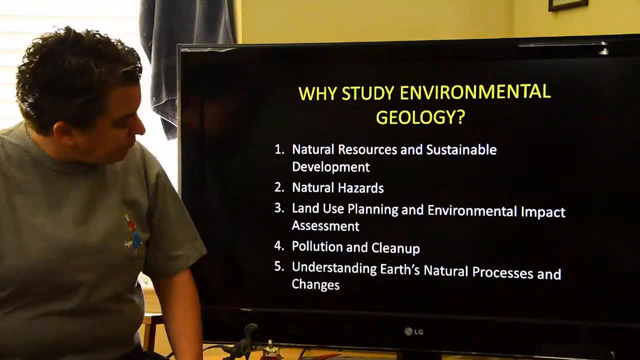 these sorts of things up and that's one aspect of environmental geology how do we clean up pollution that's in the environment and then the last reason you 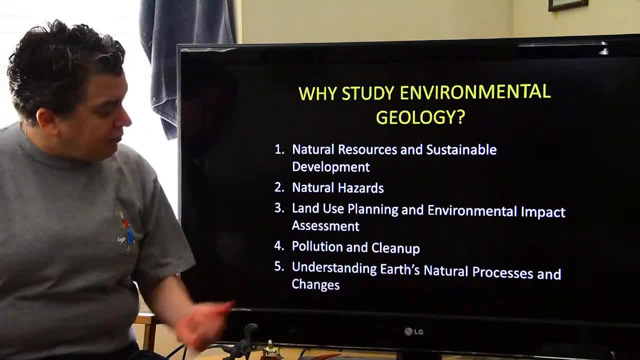 might really want to study environmental geology is just understanding 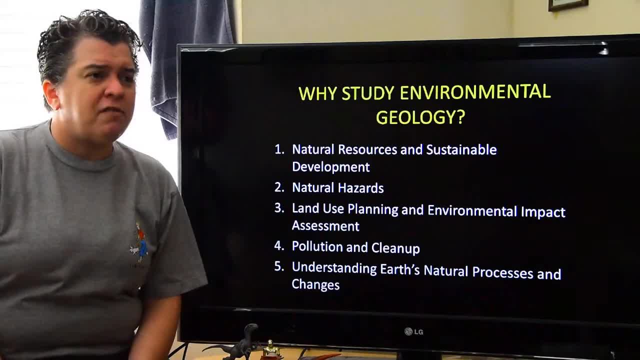 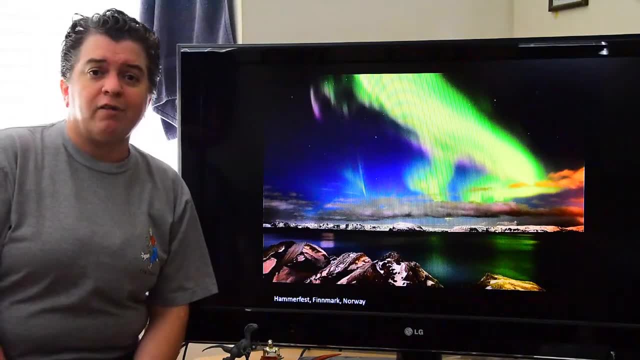 earth and the way it works and the way it changes it's kind of this natural curiosity of why do certain things happen I didn't have a really good picture for that so I just put a nice Northern Lights picture there but you 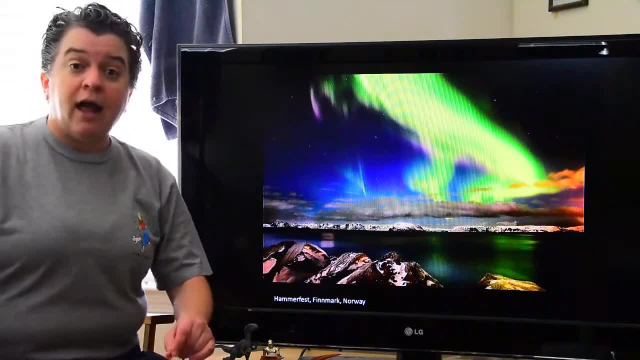 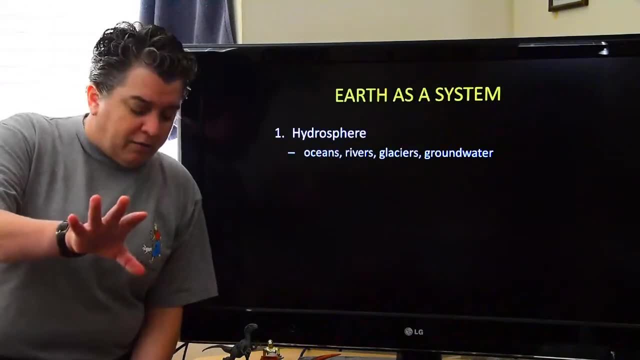 might be like why does that happen how does that happen and guess what later this semester we're going to talk about that alright now some of you guys I know 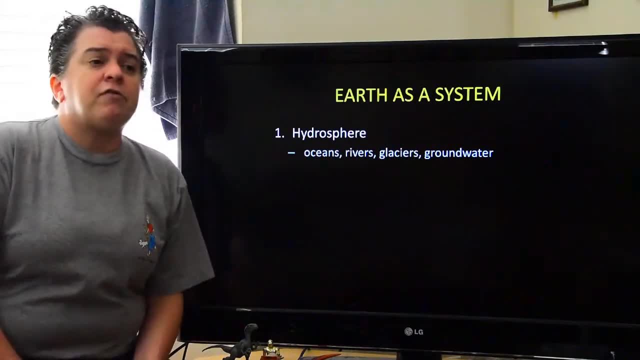 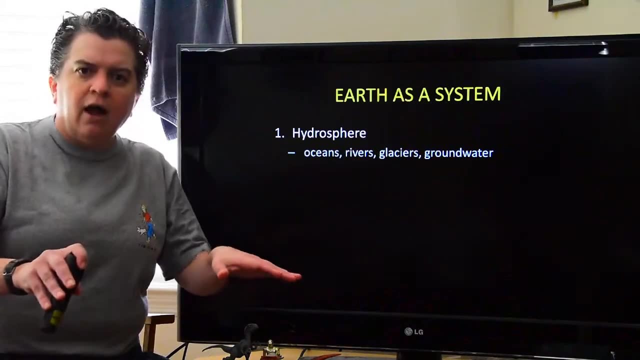 have taken physical geology but some of you haven't and so just to make sure we're starting at the kind of the same level I'm going to have a quick review 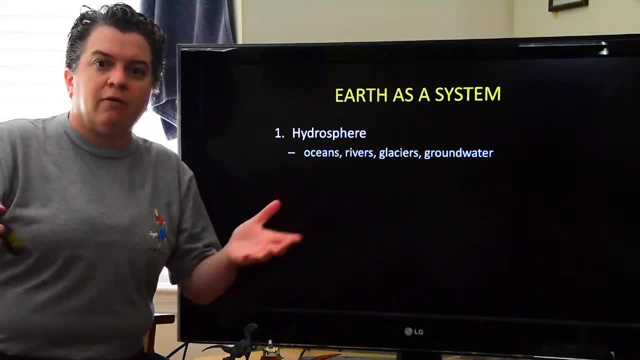 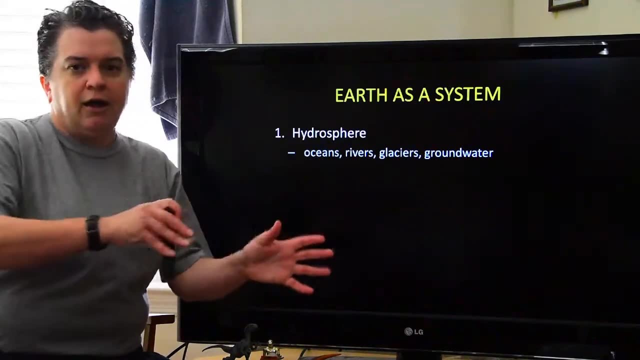 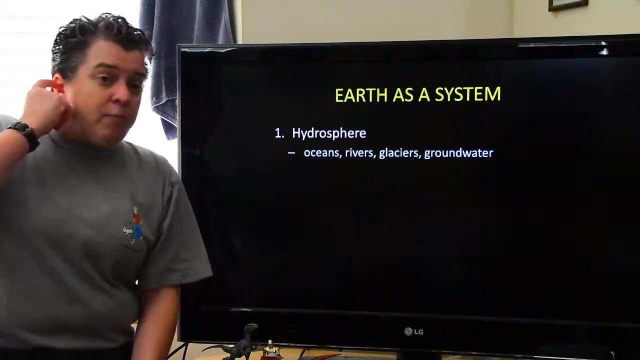 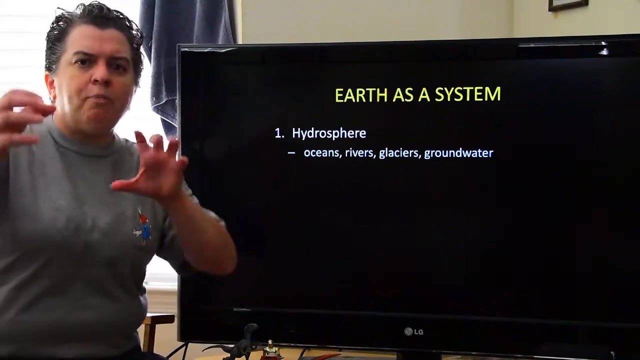 or introduction to kind of to Earth and so if you have taken physical geology this is like the review of Earth and if this is your first geology class ever hey welcome to Earth this is an introduction so one thing to remember about our planet is it's a system and when we talk about a system a system is a whole bunch of pieces that interact with each other and a change in one part 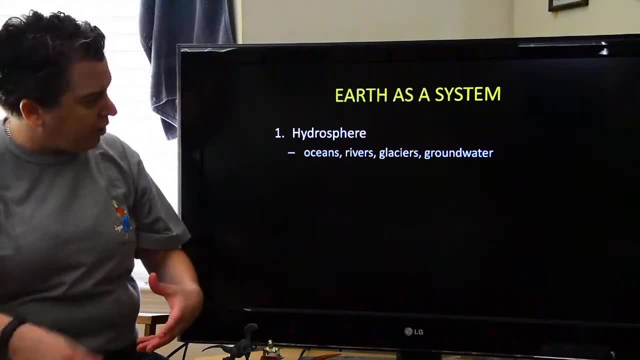 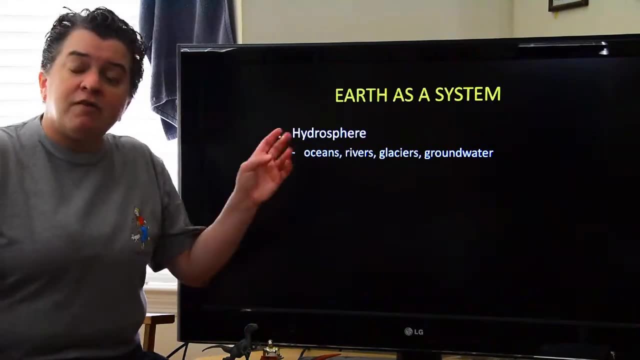 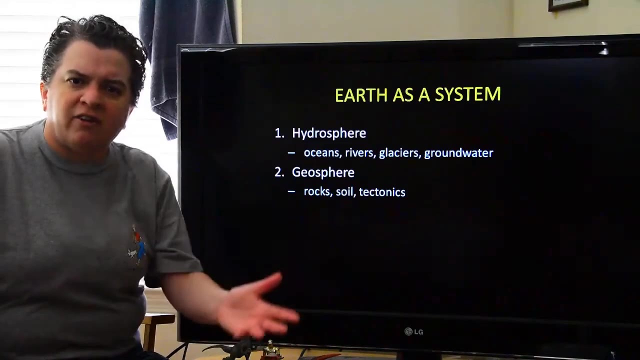 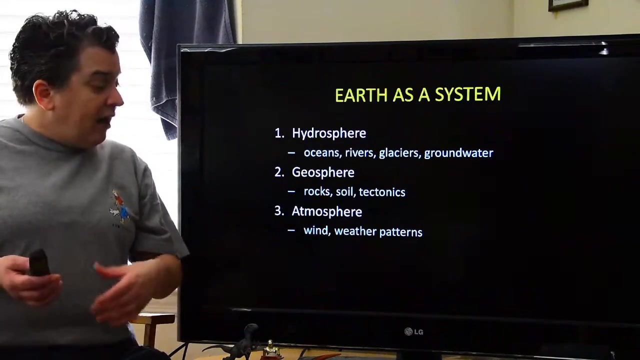 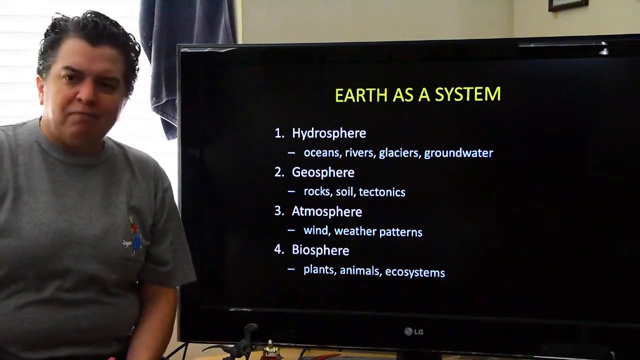 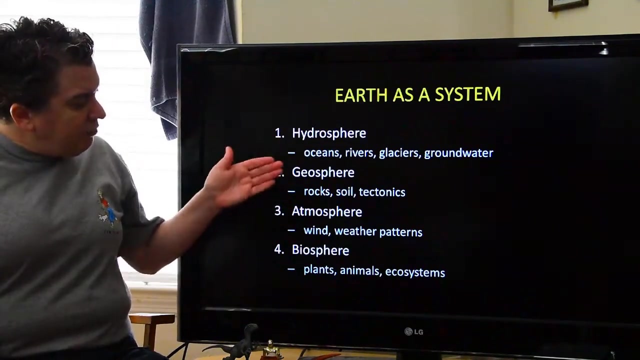 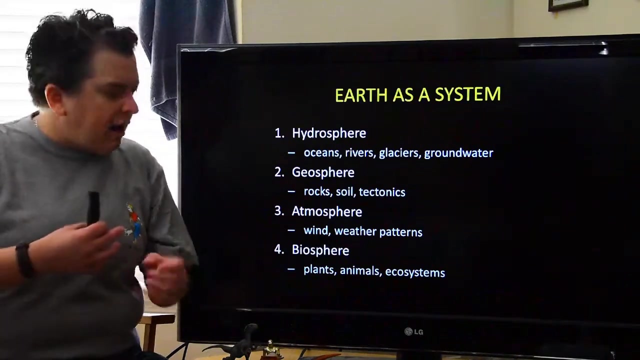 of the system can cause changes to occur in another part and when it comes to Earth there's four big parts to the Earth system we have the hydrosphere which is all of the water on the planet we have the geosphere which is basically all of the solid rock the tectonic plates stuff like that we have the atmosphere which is all of the gases surrounding the planet and that includes the winds and the weather patterns and then we have the biosphere and that's everything that's alive right plants animals ecosystems and basically each one of these can influence and change the others and so the Earth is always changing as these parts of the system are changing all 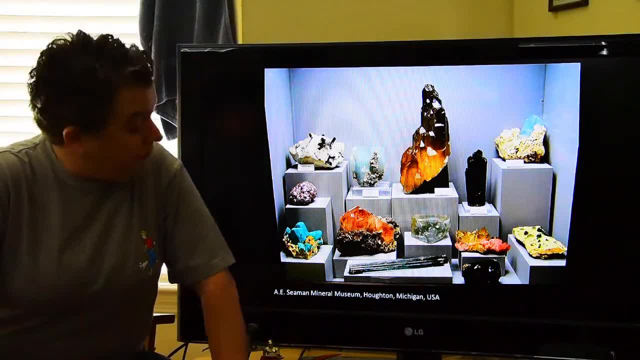 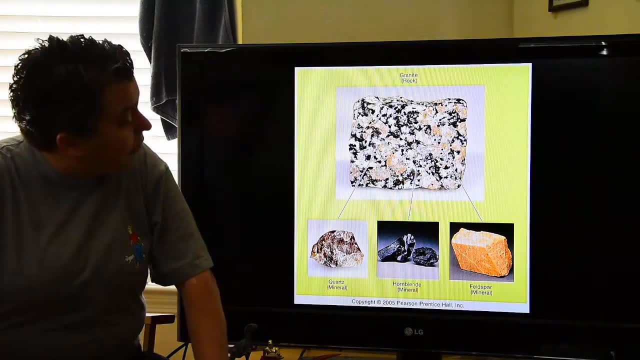 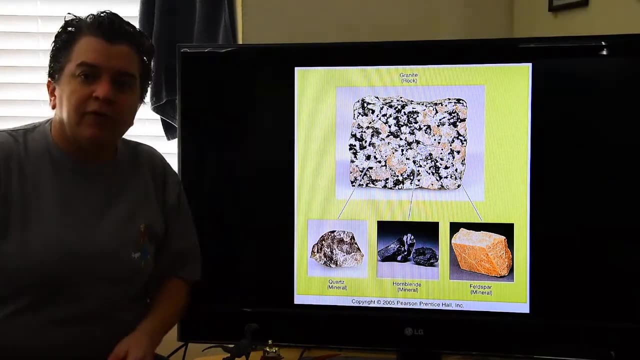 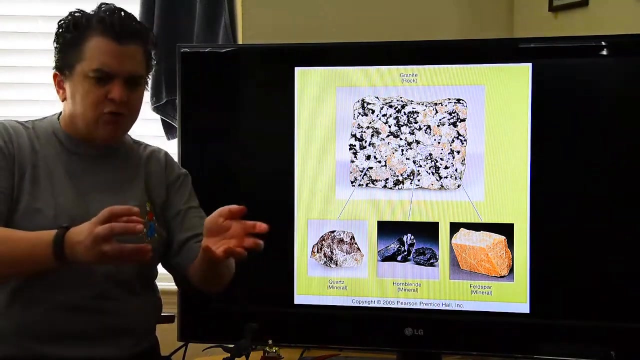 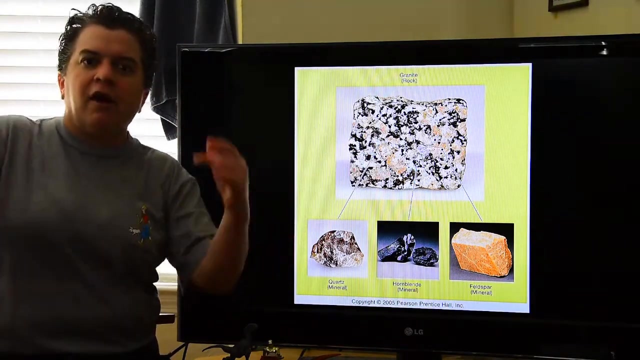 right now Earth is made up of minerals these are some pretty minerals and those minerals go into making rocks so notice in this rock this is granite we have several different types of minerals so when it comes to the physical Earth right there's atoms right and those atoms join together they combine with each other and they make minerals minerals combine with each other and make rocks and rocks are basically what our planet is made of and that's what we're going to talk about in our next lecture. 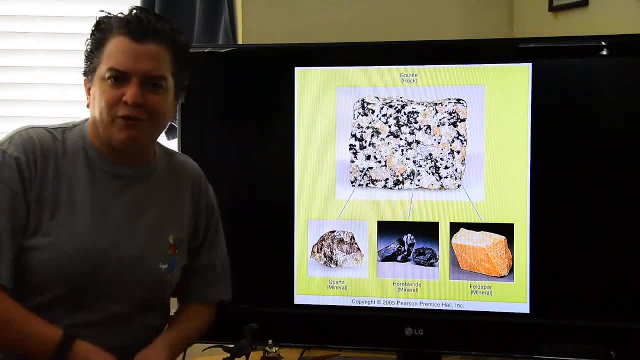 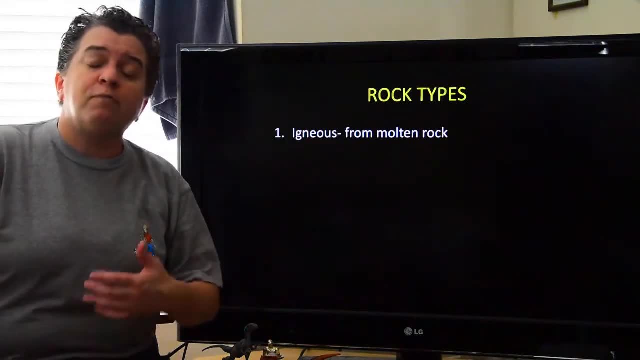 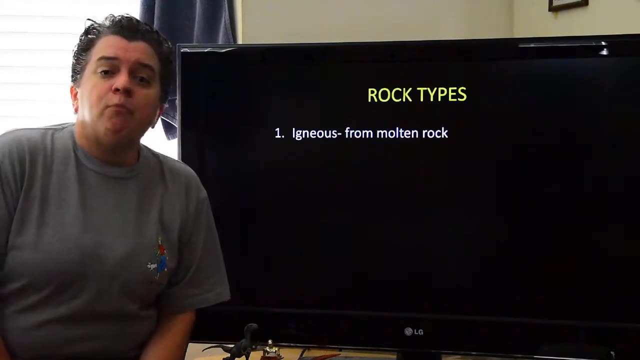 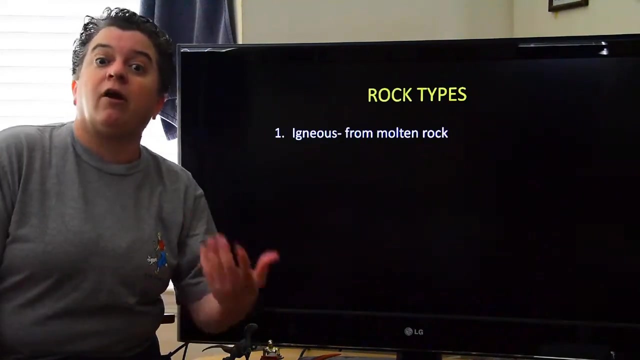 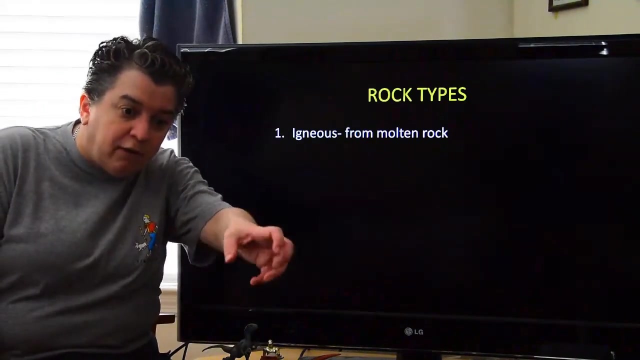 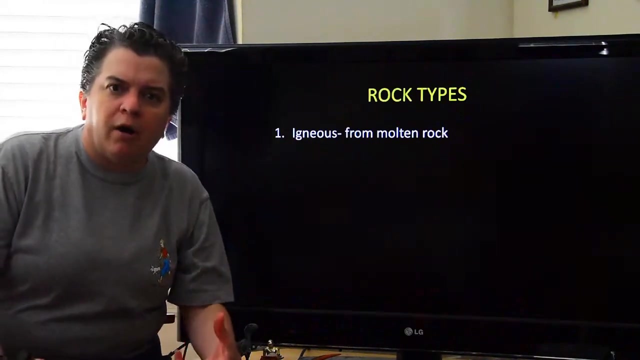 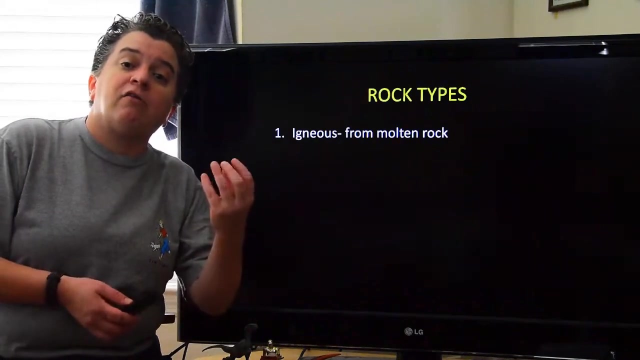 that's a quick introduction to that there are three rock types and they can behave in different ways because they were created in different ways so you have igneous rocks and these form from molten rock basically you have liquid rock that cools down and freezes right it becomes solid and this can happen on Earth's surface we see that at lava flows where the lava is moving and then it slowly cools and becomes solid this can also happen deep underground igneous rocks the the magma the liquid rock didn't make it all the way to Earth's surface in a volcano but it cooled and it became solid deep underground so igneous rocks no matter where that happens on the surface or underground they started out as liquid rock that cooled and became solid we 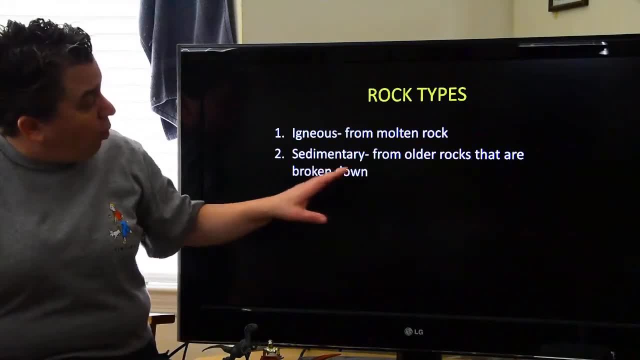 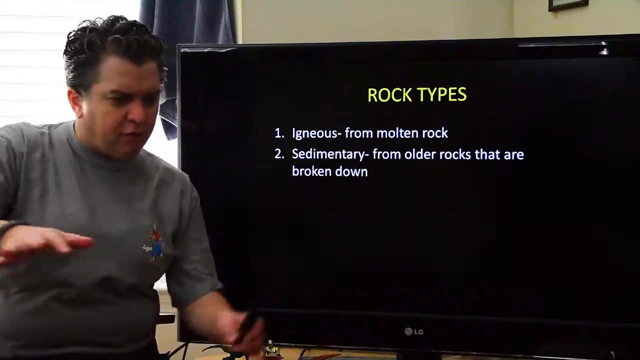 also have sedimentary rocks sedimentary rocks come from older rocks that are basically broken down and this these form at Earth's surface so at Earth's surface we have all these older 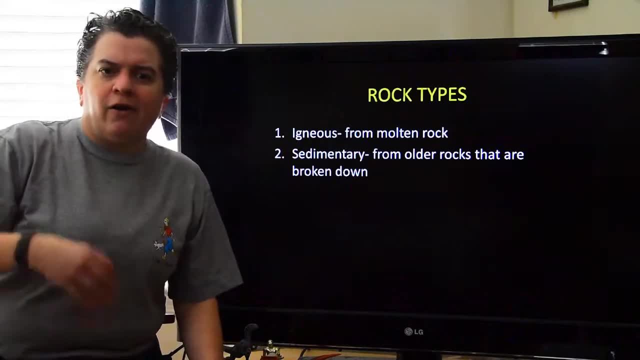 rocks and they they have rain falling on them snow plants growing in them and 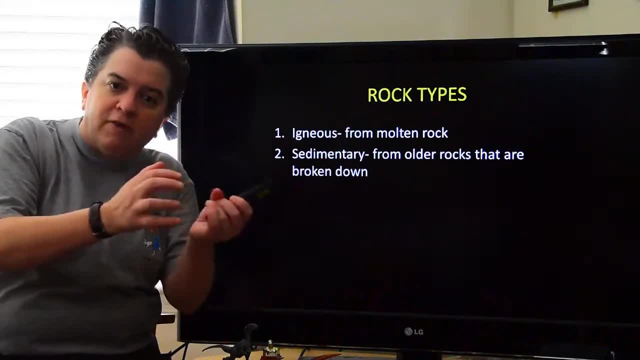 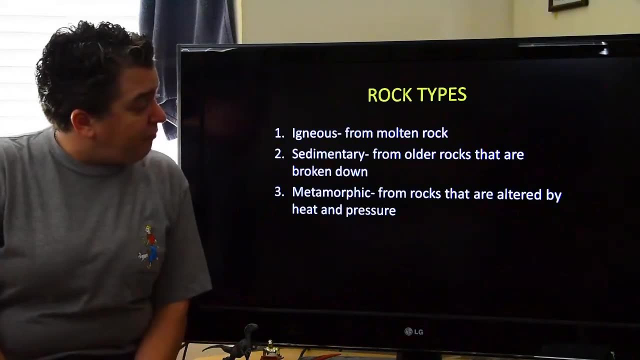 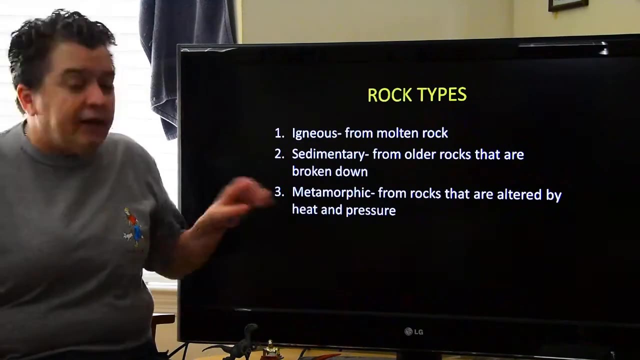 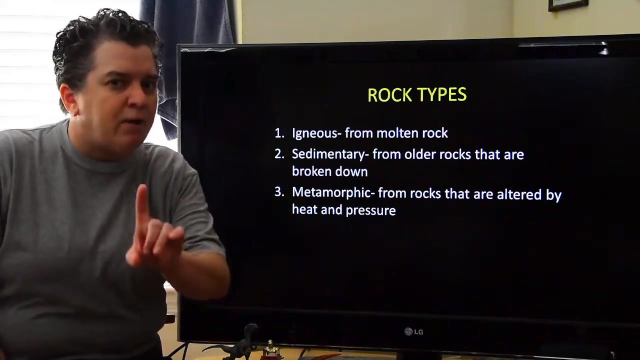 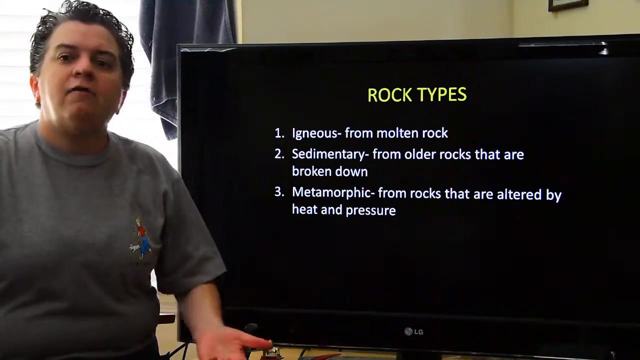 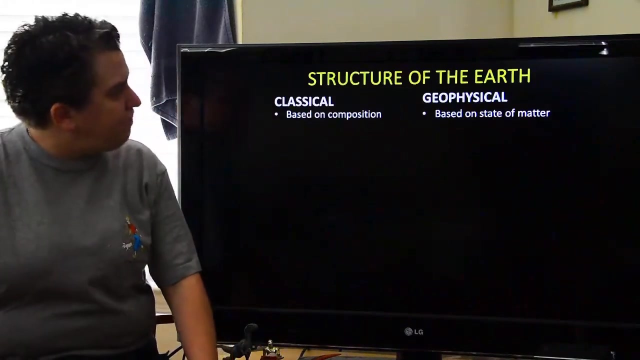 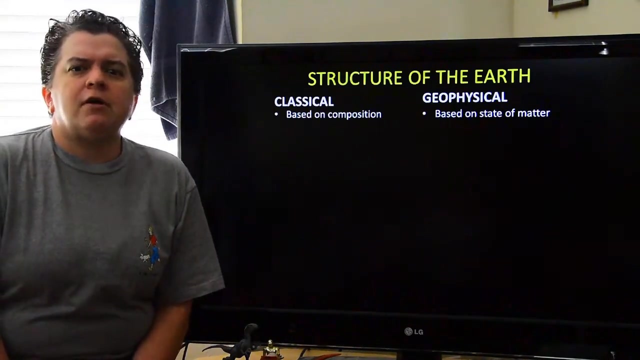 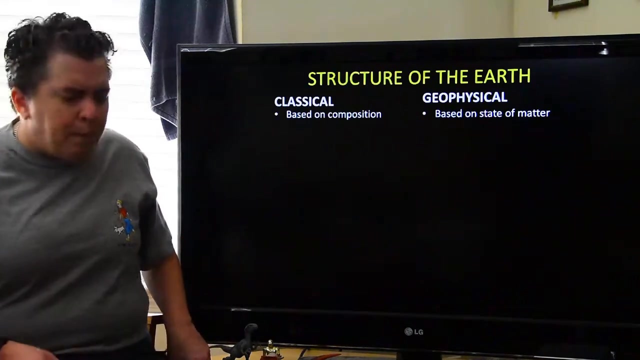 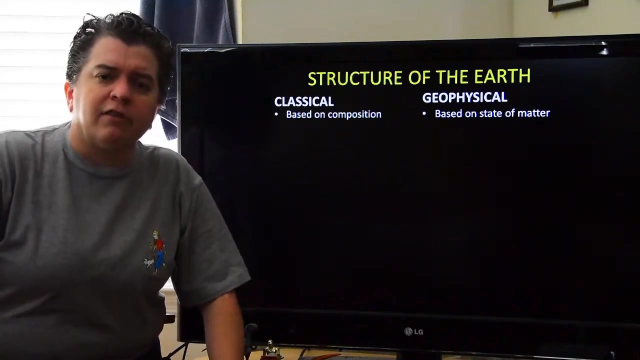 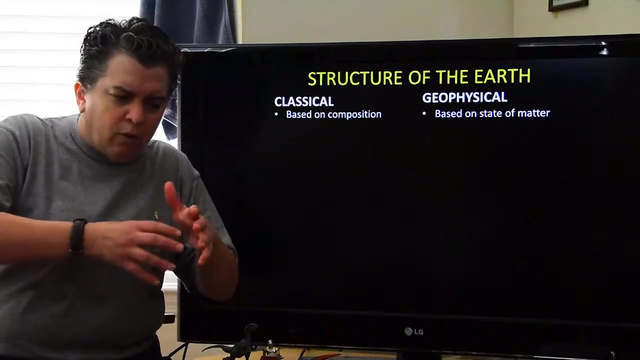 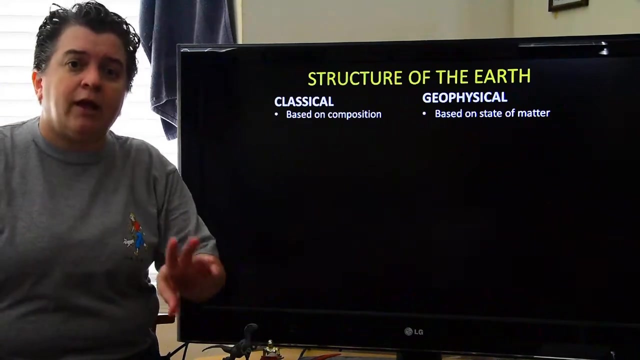 they kind of break apart those older rocks and those little bits and pieces eventually come back together in a new rock that's a sedimentary rock then we have metamorphic rocks these are formed for there from older rocks that are all altered they're changed because of high heat and pressure inside the planet high heat and pressure high enough to change them but not melt them because if they melted they'd be an igneous rock so we have these three different rock types that behave in different ways and throughout the semester I might explain you know some of the different ways these things behave all right in order to understand why rock is so important to us we need to understand why rock is so important to us we need to know the structure ofey for instance earthquakes happen and volcanoes and things like that we have to understand the basic overall structure of our planet our planet has layers like ogres have layers and the what these layers are made out of or how they behave affects the way our planet works there's two ways